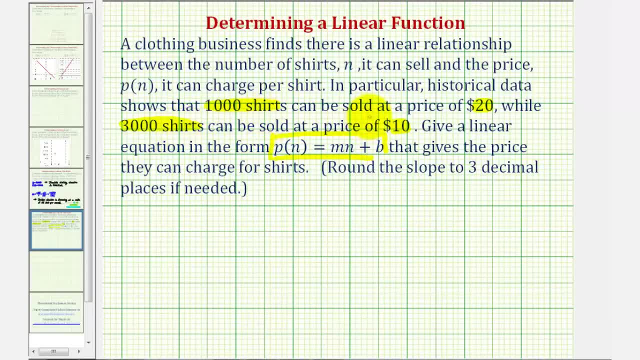 So, going back to the data, one thousand shirts can be sold at a price of twenty dollars. So one ordered pair would be one thousand comma twenty Again, where the first coordinate would be N- the number of shirts- and the second coordinate would be P or P of N. 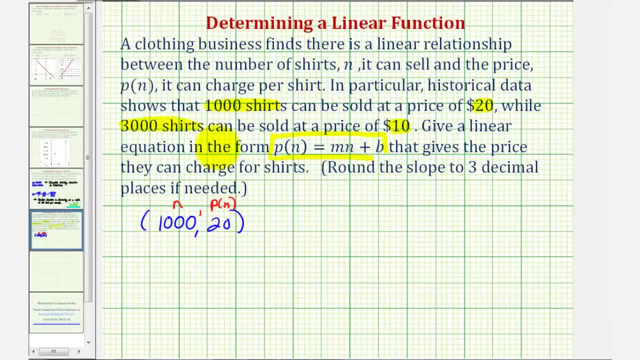 for the price. And then three thousand shirts can be sold at a price of ten dollars. so the second ordered pair would be three thousand comma ten. And now to find the linear function, we need to determine M, the slope of the linear function. 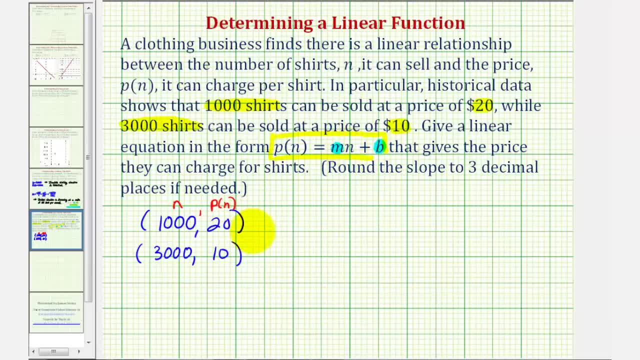 and B the y-intercept. Let's start by determining the slope using these two ordered pairs. The slope is normally equal to the change in y divided by the change of x, but in this case it would be the change in P or the change in price. 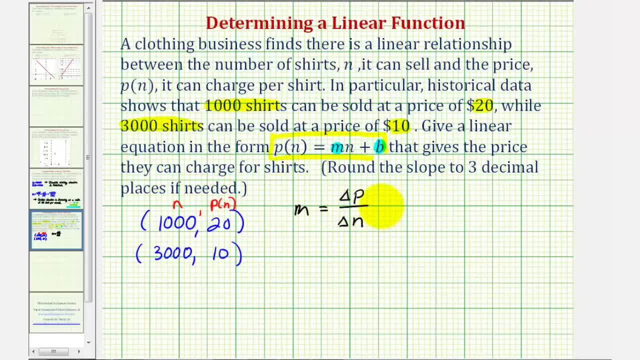 divided by the change in N, the number of shirts, Well the change in the price would be ten dollars minus twenty dollars, or ten minus twenty divided by. if we did ten minus twenty here, we have to do three thousand minus one thousand. 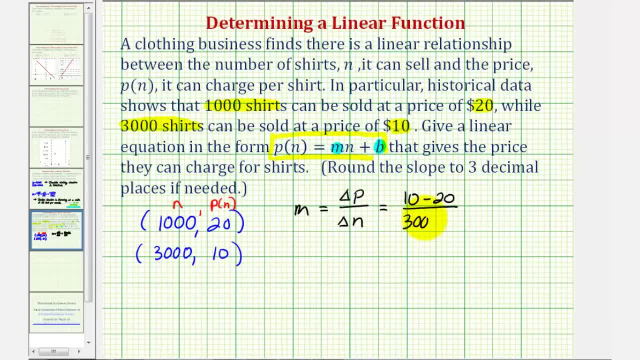 to determine the change in N. So three thousand minus one thousand, this would be equal to negative ten divided by two thousand. So our slope M is equal to negative zero point zero zero five. Negative ten divided by two thousand is equal to negative zero point zero zero five. So now we're halfway there. 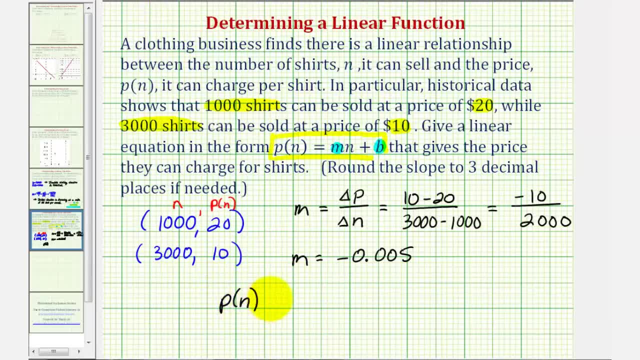 We now know that our function P of N must be equal to negative, zero point zero, zero, five times N plus B, where B is the y-intercept. So now what we'll do is select one of these ordered pairs and perform substitution for N and P of N. 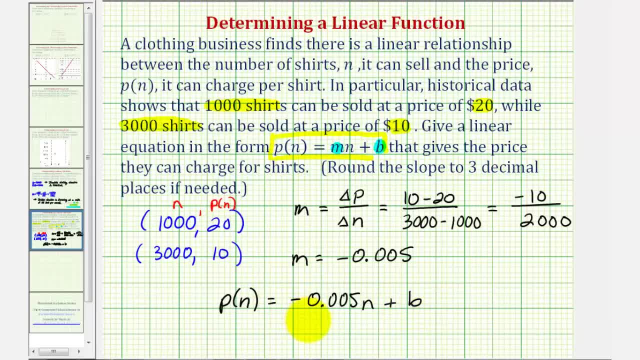 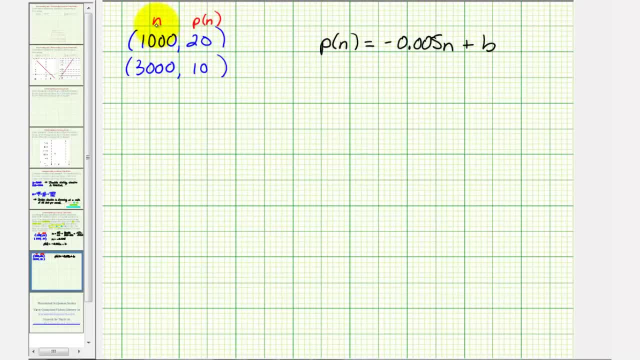 to determine the value of B. Let's go ahead and do this on the next slide. It doesn't matter which ordered pair we use. let's go ahead and use this first ordered pair. So we'll substitute one thousand for N and twenty for P of N.